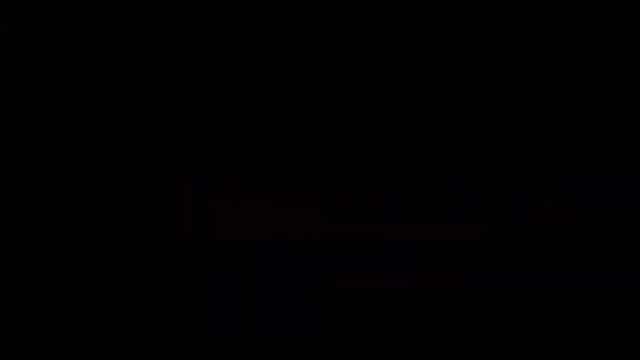 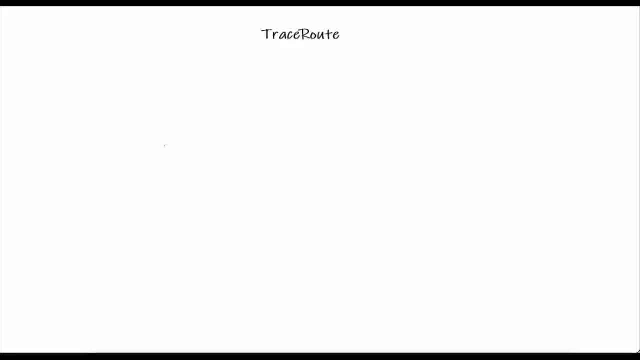 Hello everyone, welcome back to Tech Cloud channel. In today's class we are going to discuss about Traceroute. So Traceroute is basically a service or tool that track a journey from one computer to other computer. It's a service or tool. Whatever. the amount of time it takes is measured. 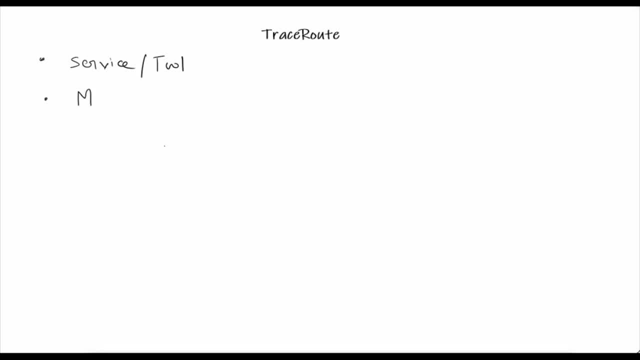 in milliseconds. Whatever the amount of time it takes to reach from source to destination is calculated in milliseconds. It's also worked by sending ICMP packet, So it's similar to ping. It also works by sending ICMP packets. Now, every router who are involved. 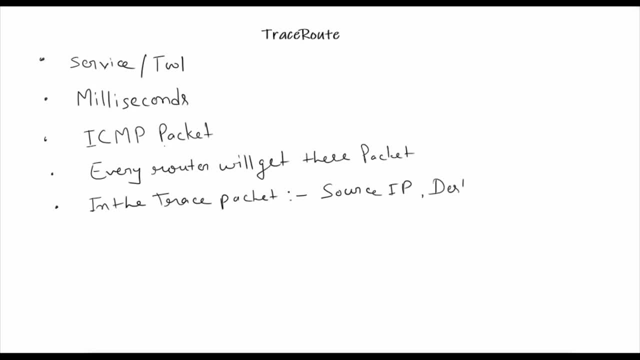 destination IP port number, so the most important in port number to know that it uses a port number range that is 33,434 to 33,534. and now it also has the message echo message. so, as we know, this dress route command, this dress route. 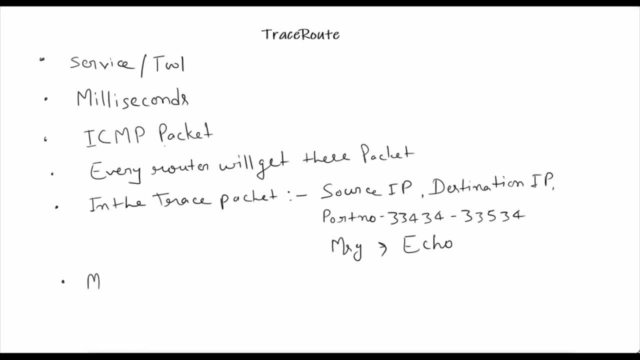 service can be used in mac machine, mac operating system, windows operating system, linux, as well as in some other open source OSS in windows. in windows the dress route send IP ICMP packet rather than default UDP packet. so the dress route behavior is to send default. it's default send UDP packet, but in windows it sends ICMP. 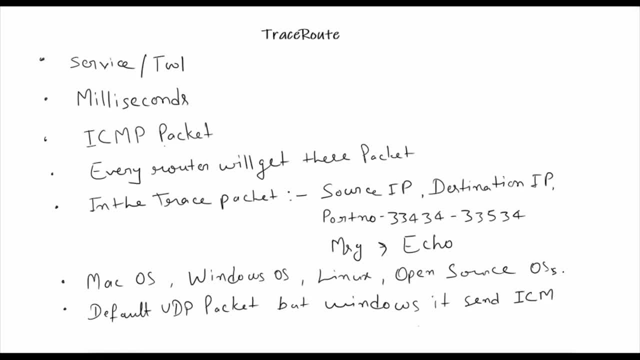 packet instead of UDP default packet. it's a tres route path. his a very enhanced version of friends. tonight we'll discuss that next works and ICMP packets- now there is some more information about trace doubts- is a very enhanced version of respect. is MTR from of MTR is mats. 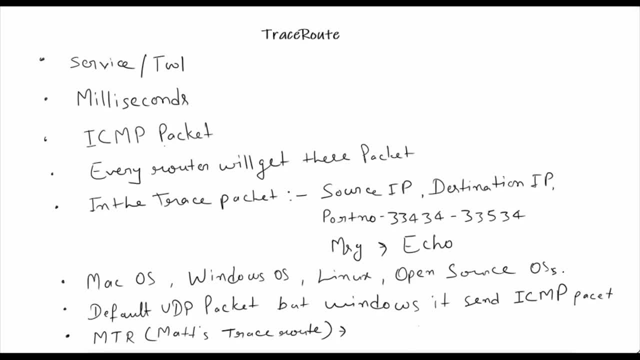 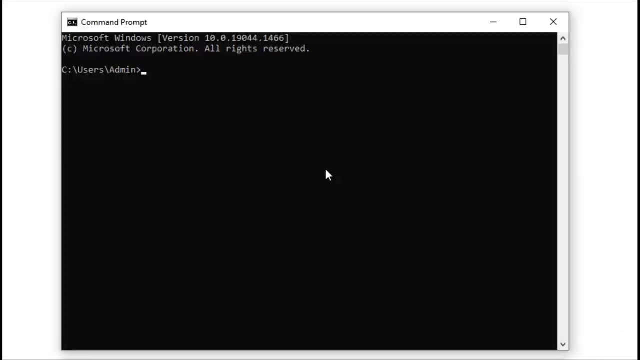 matz traceroute is an enhanced version of ICMP traceroute that is now being used in Windows and Linux both. so this is all about traceroute. now let's see how does this traceroute works, but before that let's see how a traceroute looks like. here I am tracing. 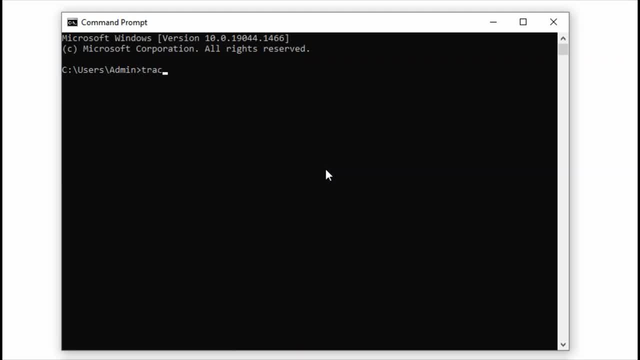 an URL that is techcloudin- traceroute- tracert. then the URL enter. this is my computer gateway now. this is my router gateway, my first gateway. now it is moving toward outside of the my router gateway. this is how it is going: from one path, one source, to other. 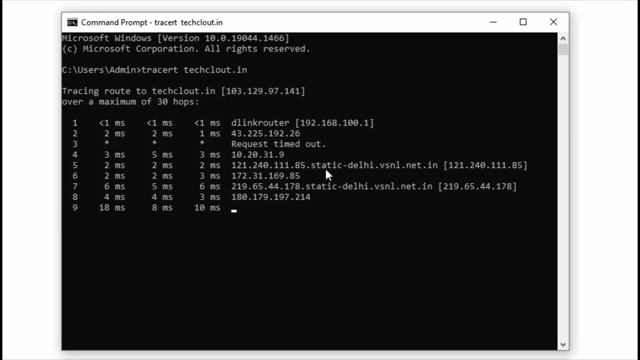 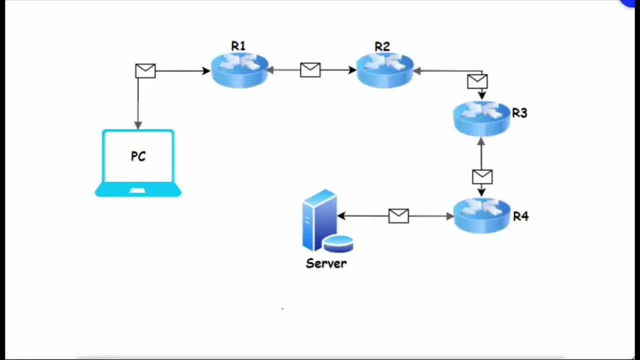 source and the destination and presenting all the hops which is coming between them. now let's move and see how does the tresserout works? okay, so now we have a diagram. in the diagram we can see there is a PC and router, one, two, three, four, and then the server. and we can see höheää 4, cái nük award. there in the diagramέςu beschgroene 1, 2, 3, 4 and then the server. 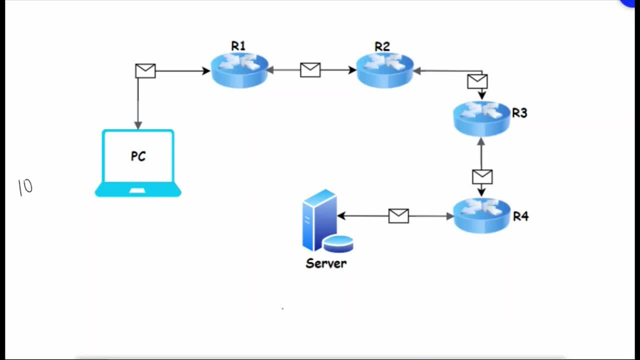 now let's see. this PC is having an IP address 10 dot 1 dot 1, dot 1 and the server IP is 2 dot 2, dot 2, dot 2. now this PC is trying to trace route. this way, PC will run a trace route command. what will happen? a echo message will be. 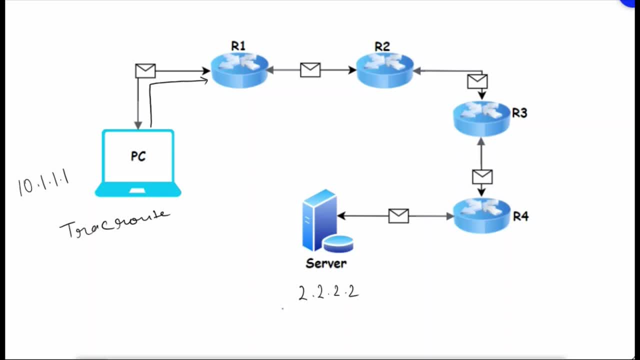 forwarded from PC to router 1, similar to the from PC to router 1. the router 1 will send same echo packet to router 2. router 2 will do the same thing, router 3 to router 4 and then router 4 to the server. everyone will send echo message. 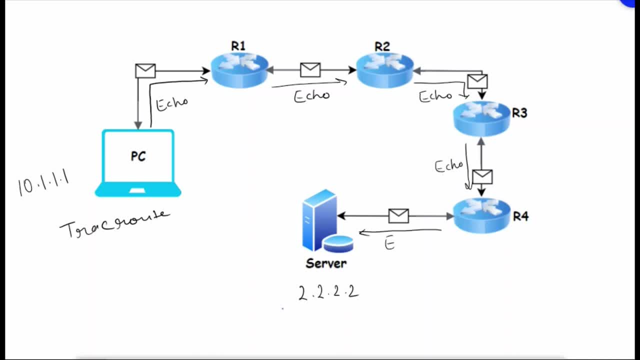 to others. now the server will reply back on echo message. that will called as echo reply. router 4 will reply back to the router 3, router 3 will reply back to router 2 and router 2 will reply back to router 1 and router 1 will reply back to PC everyone.